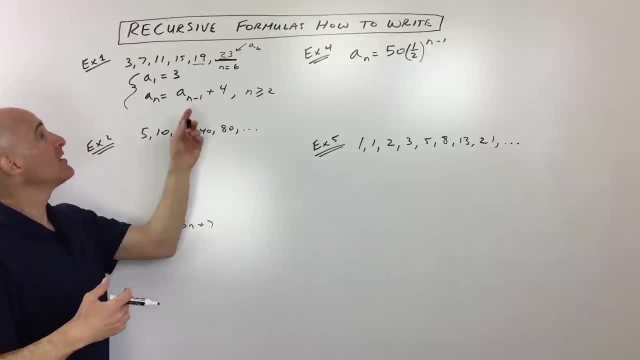 just to go one term back. you know one term before add 4 and repeat. So if I want a sub 7, I go to a sub 6, which is c7 minus 1, a sub 6, the one before plus 4 more, and I get 27.. And you keep. 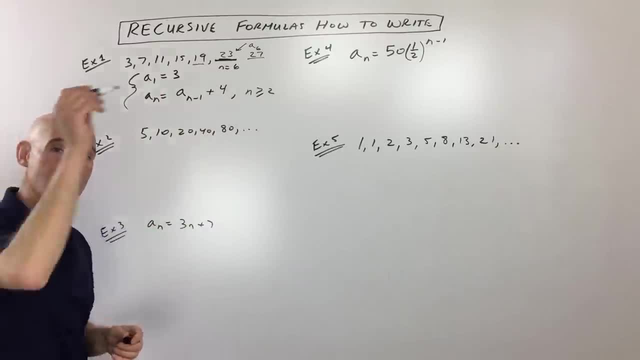 going like that. So this is different than an explicit formula where you can just put in a hundred and it takes you to the hundredth term. These are recursive formulas which are good for computers And you can write a little program and it'll keep you know, taking that previous term and 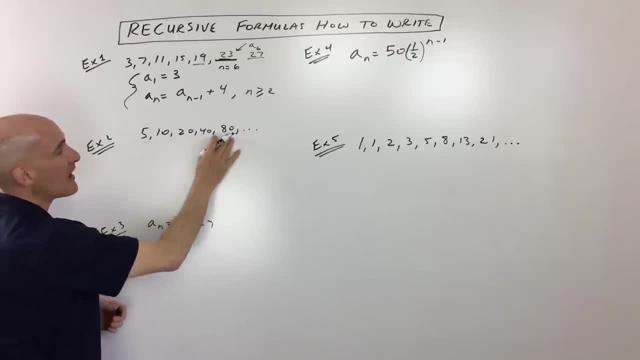 repeating. So let's look at example number two. What's the pattern? How are they getting to the next term in this sequence? Can you see What are they doing to get to the next one, next one, next one. Okay, well, if you said multiplying by 2, you're absolutely right. The first term, a sub 1. 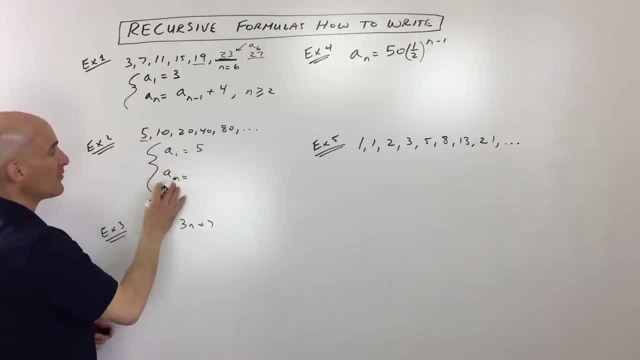 is 5, right. And then if we want to write a formula to get to the value of the a sub nth term, you just take the a sub n minus 1th term, the one before, and then you multiply by 2.. And that's for when n is greater than or equal to the second term. 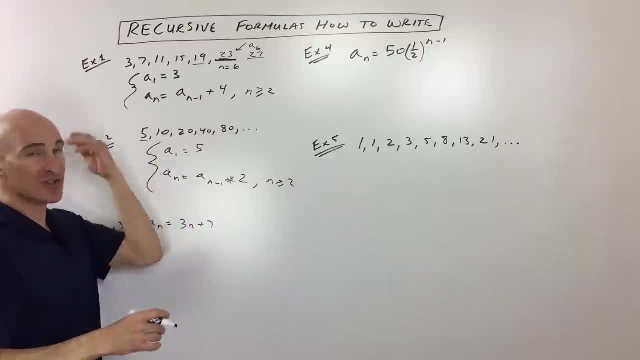 You know. so this wouldn't work if you know you were at the first term, because we really don't know what the zeroth term is right, So that's the idea. So you just take the previous term, That's what this, a sub n minus 1, represents, And then you tell the person how do you get to the? 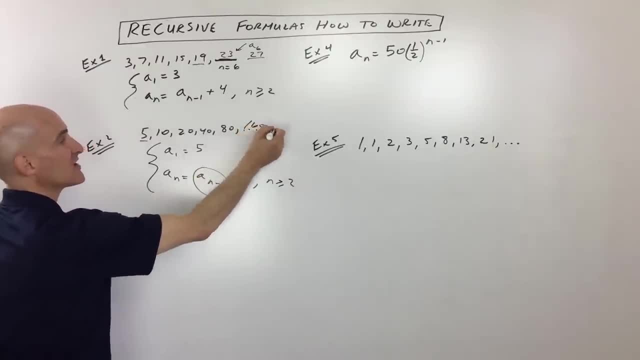 next term. Oh, you just multiply by 2. Okay, So 160 and so on. Okay, The third example: they're giving us an explicit formula. They're saying: you know, if you want to find the hundredth term, 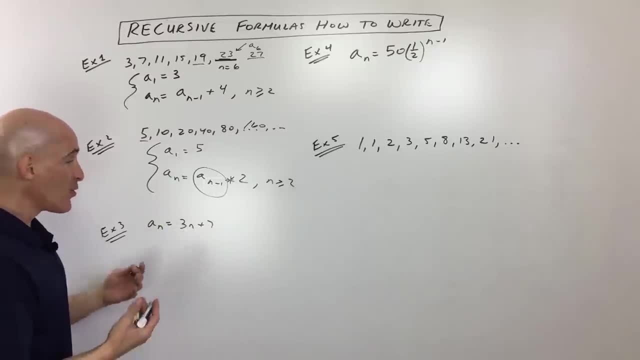 you put in a hundred, that's going to be 307.. But we want to write a recursive formula, So what we'll do is just put 1 in. okay, n equals 1.. So that gives you 3 times: 1 is 3 plus 7 is 10.. 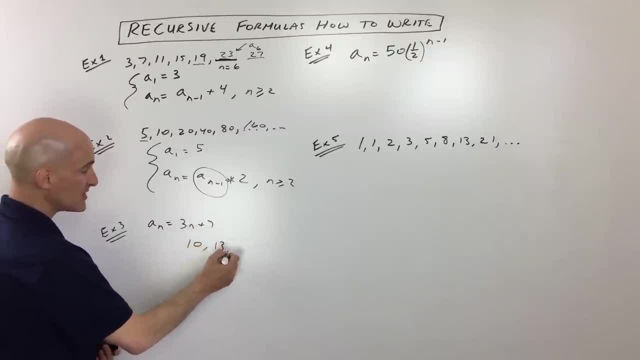 And then let's maybe put 2 in. That would be 3 times 2 is 6 plus 7 is 13.. And let's put 3 in, and that gives us 16, and that gives us 19, and dot, dot dot. So now you can see the pattern. 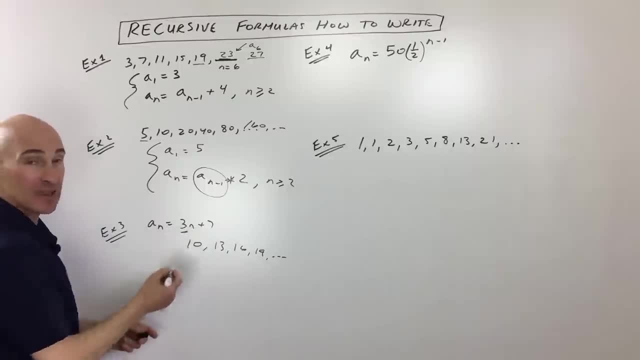 It looks like we're adding 3, which makes sense, because see how this is like a line like: y equals 3x plus 7.. You know the slope is 3.. It's increasing by 3.. But if you want, you can write. 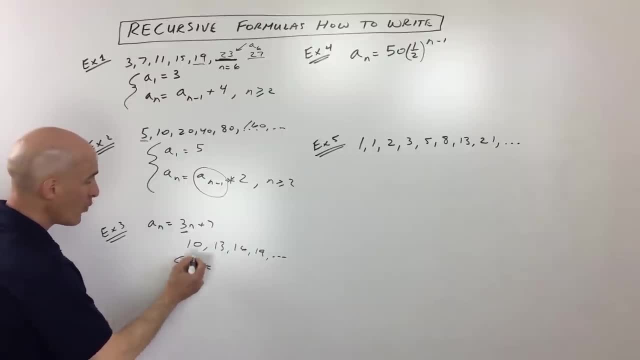 out a few terms- A lot of students like to do that method- And then a sub 1 is the value of the first term, which is 10.. And then what we want is a formula to find the next term in the sequence: You take the previous term, a sub n minus 1, and you add 3.. And then this is just 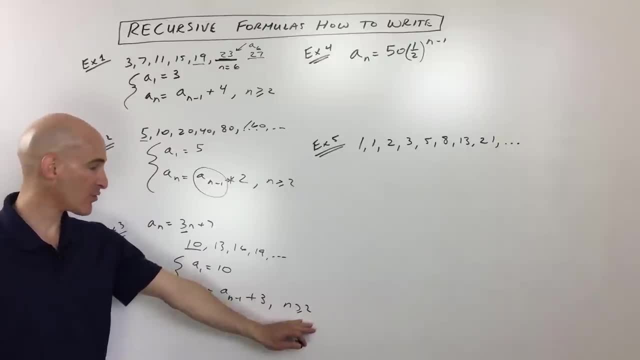 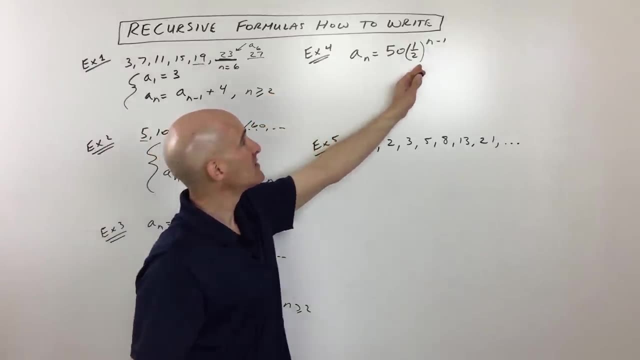 for when n is greater than or equal to 2.. Some teachers don't really worry about having you write this, but I'm just showing you that, in case your teacher does. So that's that one. Now, for example, 4, this formula also is an explicit formula and it takes you right to you know. 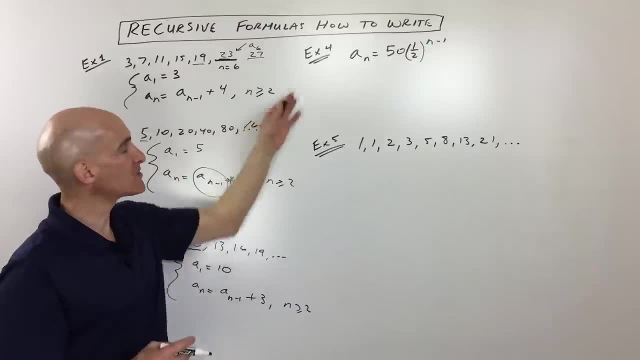 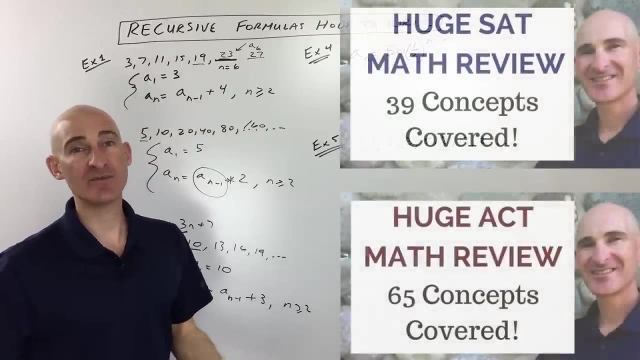 whatever term you want. If you want 100, you put in 100.. But before I get to these next two examples, I want to mention that if you're preparing for the ACT or the new SAT- the math sections- I've got two video courses to really help you boost your score on those math sections of those. 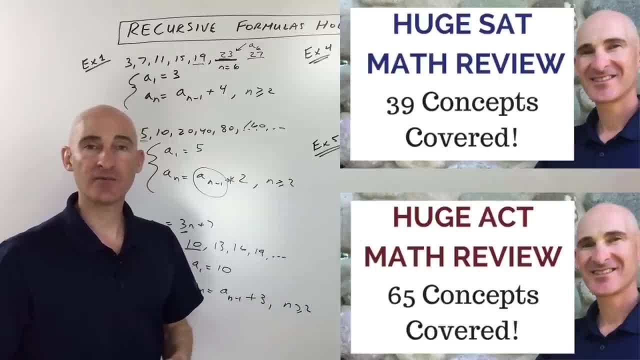 two important tests So you can check out those. I've got the description below. You can check that out, or the links on my About page. I've got links to those video courses. They're really in depth. They go through 39 concepts with the SAT one and 65 concepts with the ACT one going through. 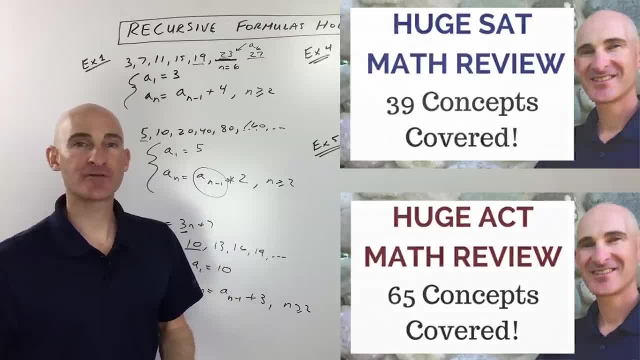 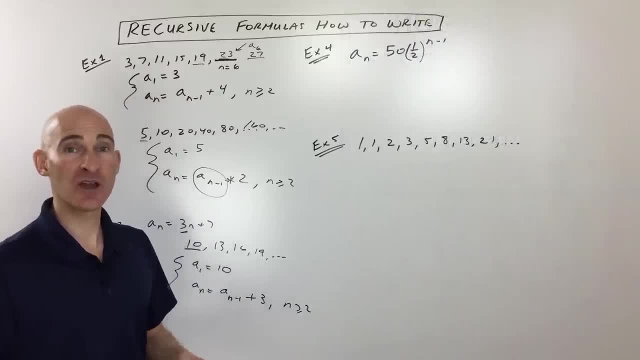 all of those. So if you're interested in taking those courses, you can go ahead and check out the free previews, And I'm sure you will, too, Check out the free previews to see if it's something that you're interested in and look into getting those courses if you're getting. 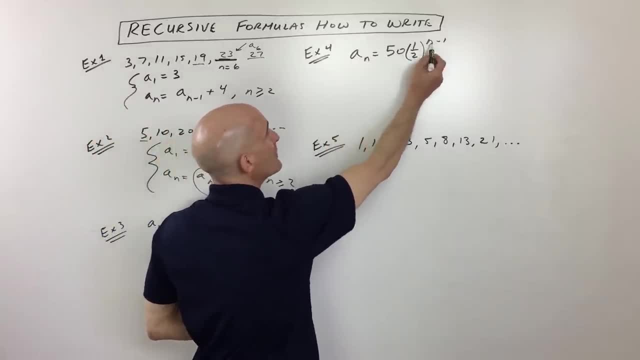 ready to take those tests. But to go back to this problem, let's just write out a few of the terms. So if I put 1 in, 1 minus 1 is 0.. 1 half to the 0 power is 1 times 50 is 50.. So our first term is 50.. 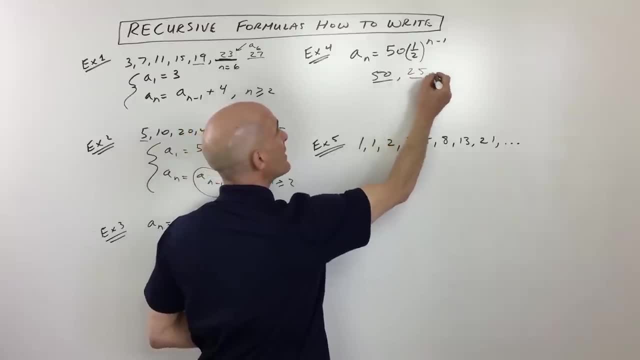 If we put 2 in, 2 minus 1 is 1.. 1 half to the first power is 1 half times 50 is 25.. And you can go ahead and look at the formula. You can see we're off and running. now It looks like we're multiplying by. 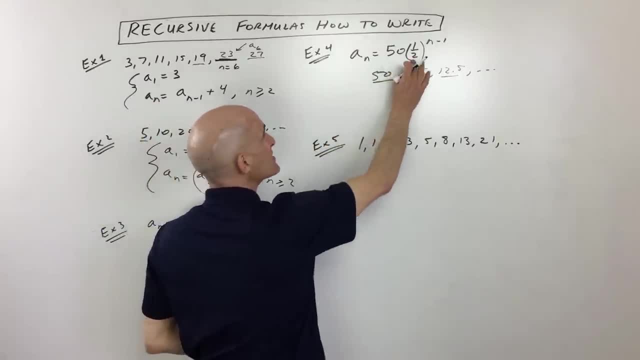 a half each time. Now, if you're already familiar with the explicit formula, you can see this is your ratio. So that's what we're multiplying by- And this is your first term- a sub 1.. But just to show you, in case you get stuck, you can always put in a few terms: starting with n equals 1 to. 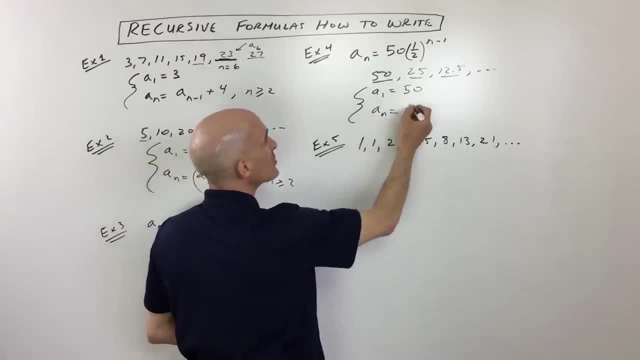 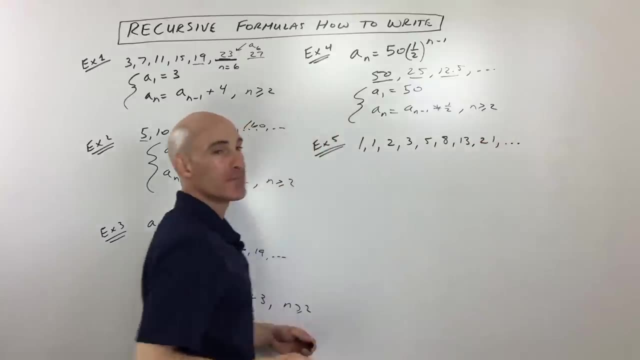 find the pattern. But now what you can see here is what we're doing is we're taking that previous term and we're multiplying by a half, And that's for when n is greater than or equal to 2.. Okay, let's look at another example. This is a famous sequence. It's the Fibonacci sequence. You've 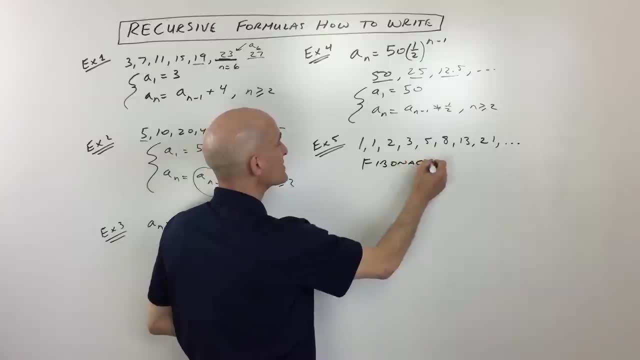 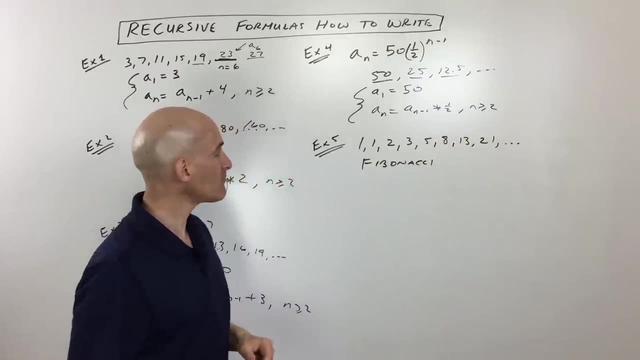 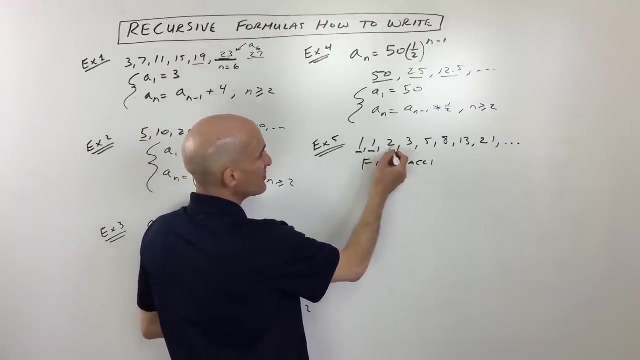 probably heard about this before or maybe learned about it earlier in your math classes. But see if you can see the pattern. Like: how are we getting from these terms to the next term? Can you see the pattern? Well, what's happening here is, if you can see it is that we're adding 1 and 1 together. 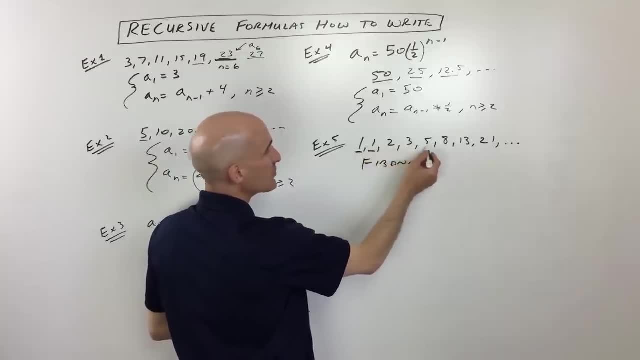 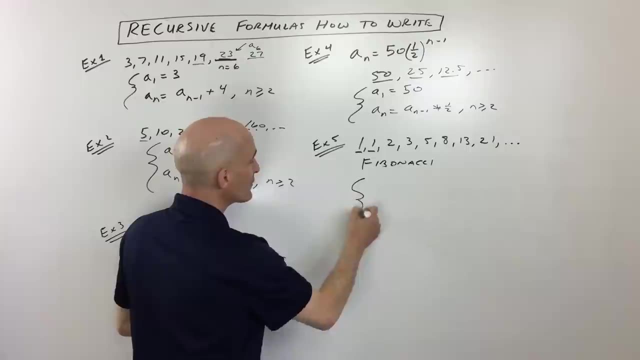 to get 2.. We're adding 1 and 2 together to get 3.. We're adding 2 and 3 together to get 5.. Basically, what we're doing is we're adding the two previous terms together to get the next term. So what I'm going to do for this one is I'm going to say that a sub 1 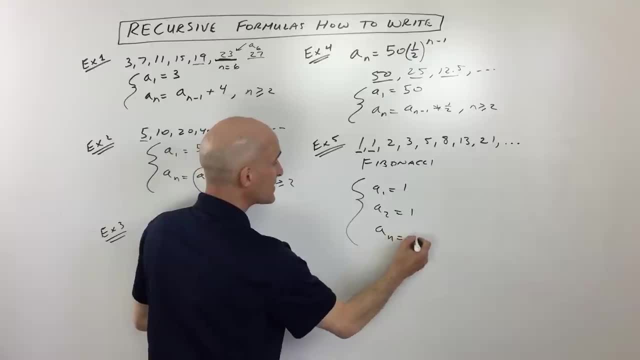 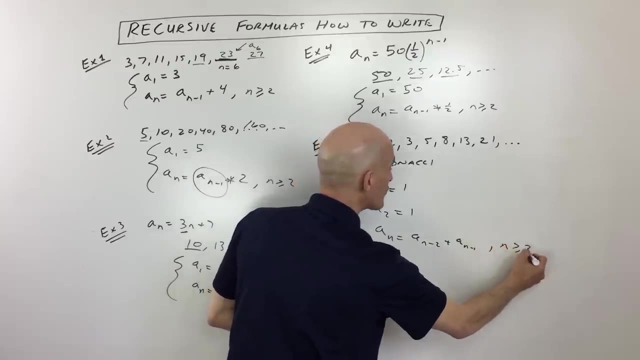 is equal to 1.. a sub 2 is equal to 1.. a sub n is equal to a sub n minus 2 plus a sub n minus 1.. And this is for when n is greater than or equal to 3, meaning the third term and beyond. 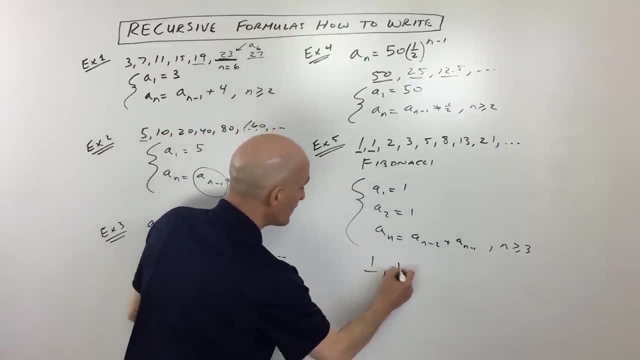 right. So they're giving us the first two terms, see 1 and 1.. If we want to find the third term, we go to the 3 minus 2,, which is the a sub 1th term, and then the 3 minus 1,, which is the a. 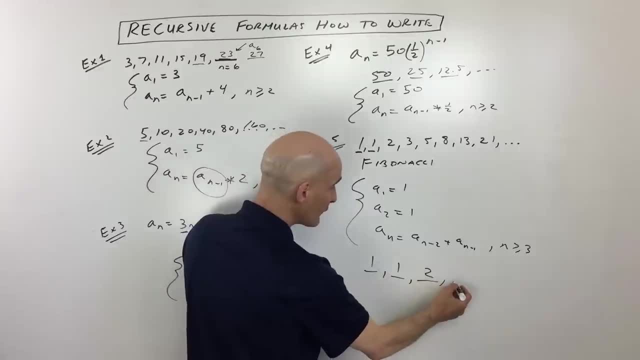 2th term And we add those together and we get 2.. If you want to find the a sub 4th term, 4 minus 2 is 2.. So we go back to the second term: 4 minus 1 is 3.. We go back to the third term. We add those. 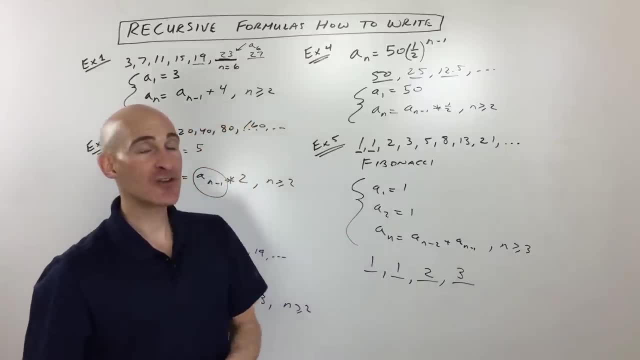 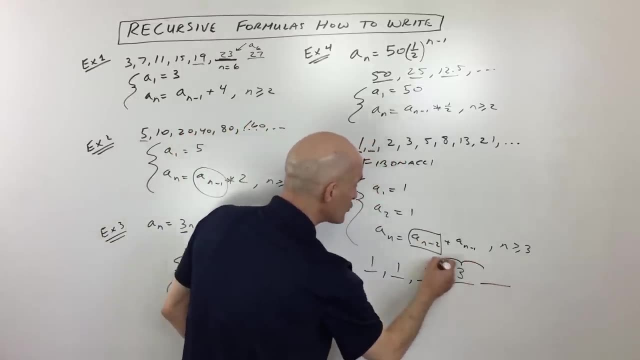 together and we get 3.. And it continues like that. But after you do this a while, you'll kind of just look at the a sub n minus 2 and just say to yourself: hmm, that just means that I go two terms back, And a sub n minus 1 just means that I go just one term back. 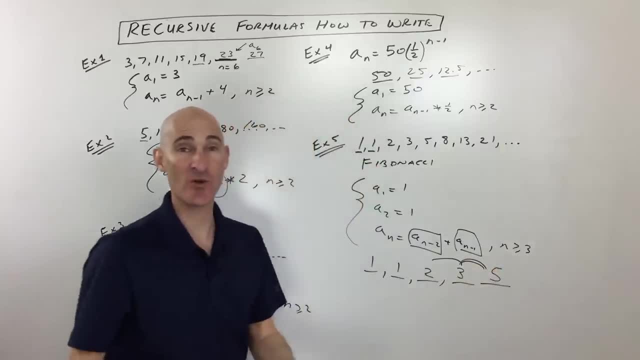 and I add those together And that's how I'm getting the next term in the sequence. So I hope this helped you understand how to write recursive formulas a lot better. Check out the more math videos that I have on my Mario's Math Tutoring YouTube channel. I have hundreds and hundreds of 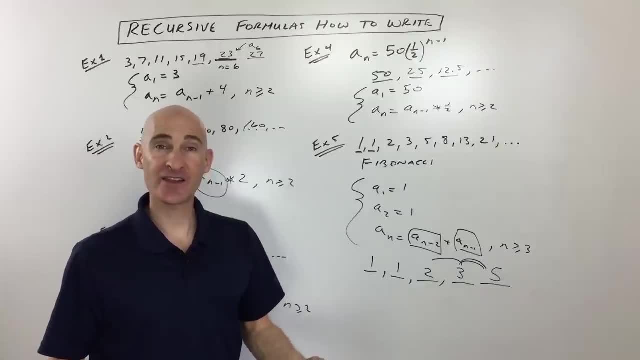 videos to help you boost your score in your math class and make learning math a lot less stressful, and just help you understand better. overall Subscribe to the channel and I look forward to helping you in the future videos. I'll talk to you soon.